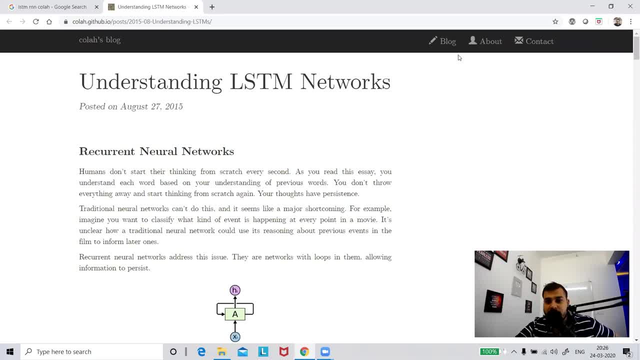 Hello all my name is Krishnayak and welcome to my YouTube channel. So, guys, today, in this particular video, we are going to discuss about LSTM- recurrent neural networks. Now, many days has been over. I have not uploaded this particular video in my deep learning playlist. 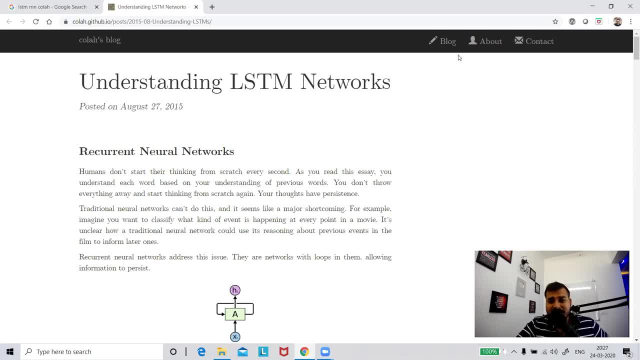 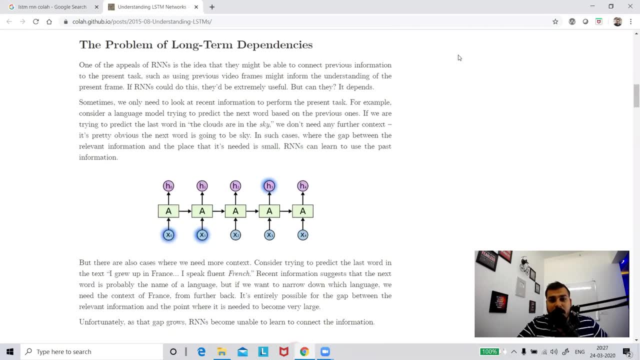 so we'll continue it and we'll try to finish it off. So I've already discussed about simple recurrent neural network. we have understood what are the problems of simple recurrent neural network. I told you that there is a problem of vanishing gradient right. 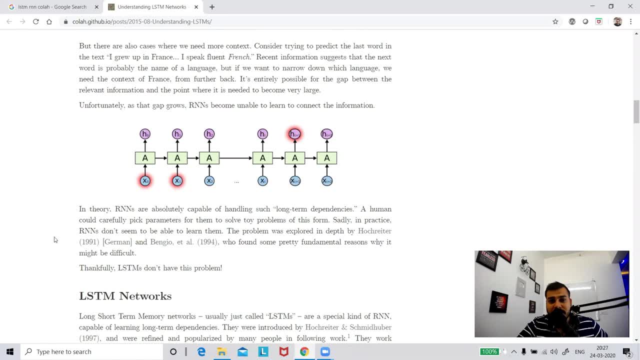 Whenever you have a deep recurrent neural network and suppose your output is dependent on one of the inputs which is there in the initial stages, so during the back propagation, there is the problem of vanishing gradient problem. that basically means when the weights are getting updated with the help of back propagation using the chain rule. 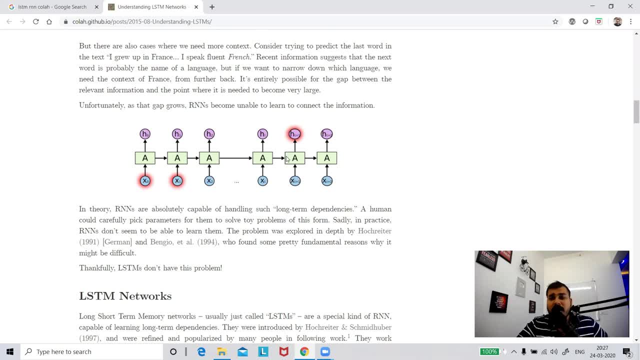 that time the weight actually becomes a very, very smaller value or the weight updation does not happen, because when you're finding the derivative of that specific weight, it will be a very small number. So if you have not seen my vanishing gradient problem, 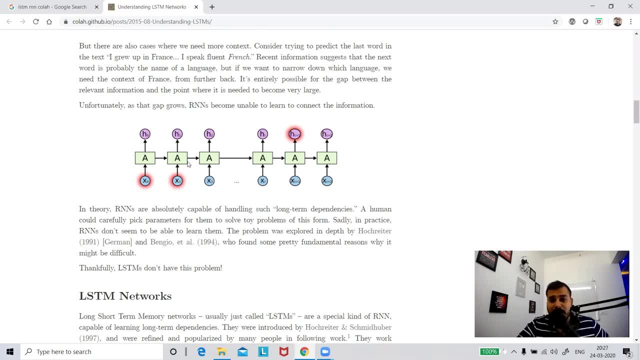 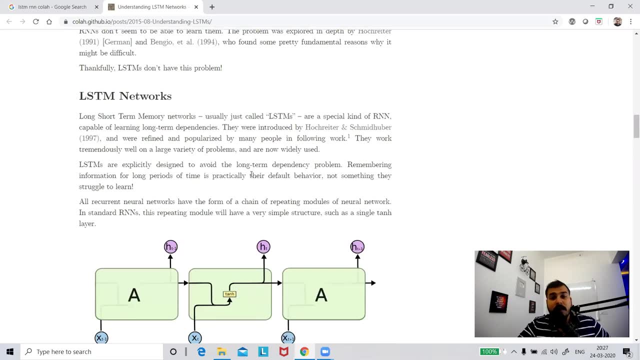 just go and watch my complete deep learning playlist. all the videos have been uploaded Now. today, in order to solve this particular problem, we basically use something called as LSTM- recurrent neural networks- and GRU. Today, in this particular video, we'll discuss about LSTM- recurrent neural network. 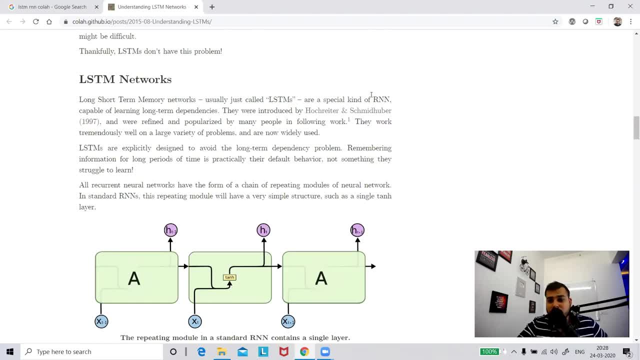 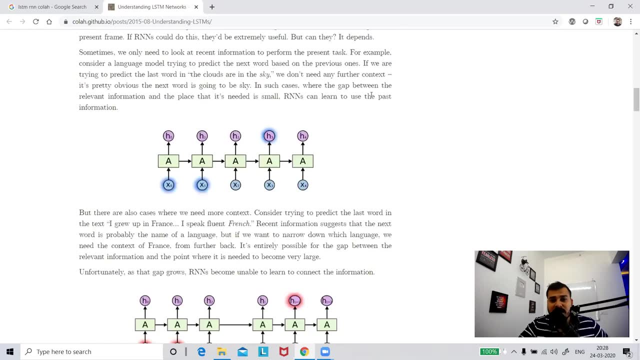 and remember, guys, please do follow this blog from Kohlhaas blog. so, Kohlhaas blog, I'll completely dedicate this particular video to this particular blog. this is a wonderful explanation and just by reading it, reading the text, you will be able to understand everything. okay. 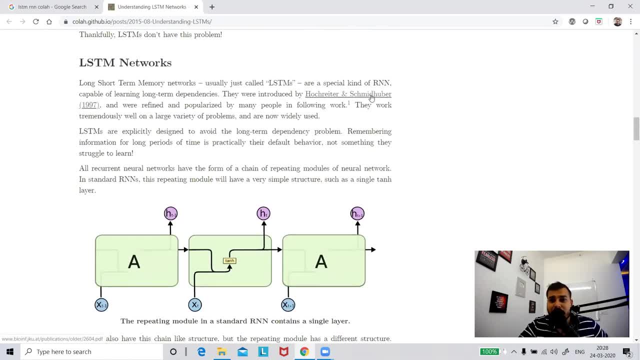 Now let us go ahead and try to understand. how does the recurrent neural network you know work? and here you can see that LSTMs are explicitly designed to avoid the long-term dependency problem, So they are actually focused on resolving the vanishing gradient problem itself. 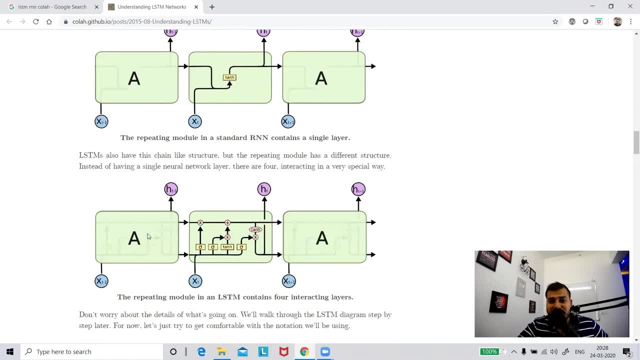 So this is how my simple recurrent neural network looks like, and this is basically my LSTM recurrent neural network looks like. Don't overcomplicate yourself by seeing so many gates, but we'll try to divide this whole architecture into some steps and then we'll try to understand that. 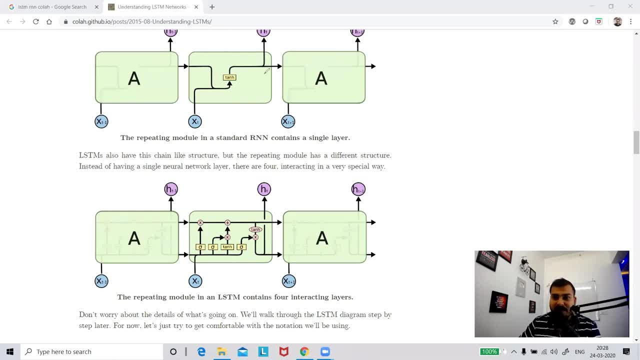 So over here, the first thing that we need to discuss. we'll divide this into various components, So the first component is basically called as memory cell. okay, We'll try to understand what exactly is memory cell. then we have forget gate, okay. 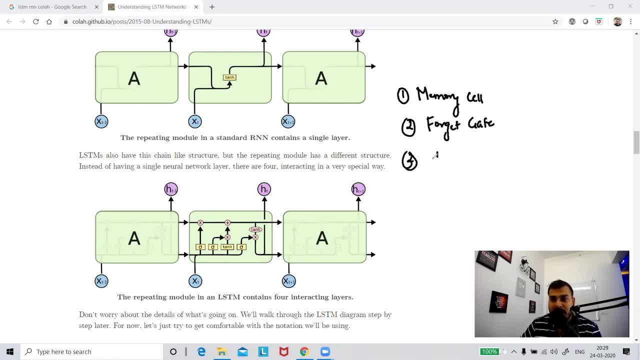 Forget gate. then we have the third thing is have we are having is something called as input gate and the fourth thing that we basically have is called as output gate. Okay, so we'll try to understand what is memory cell. So this whole part. 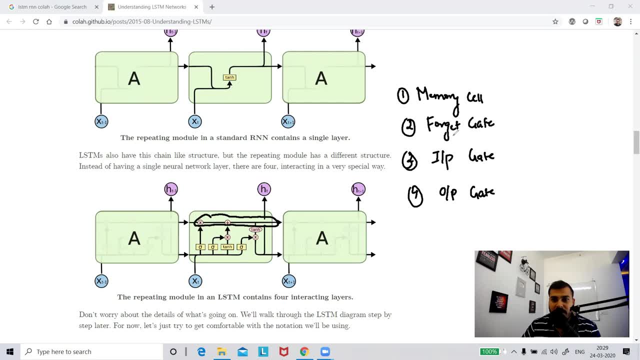 this whole part is actually called as a memory cell. okay, If I talk about forget gate the first, this particular diagram is basically the forget gate. then we have the input gate. this whole thing is basically the input gate, and then we have the output gate. 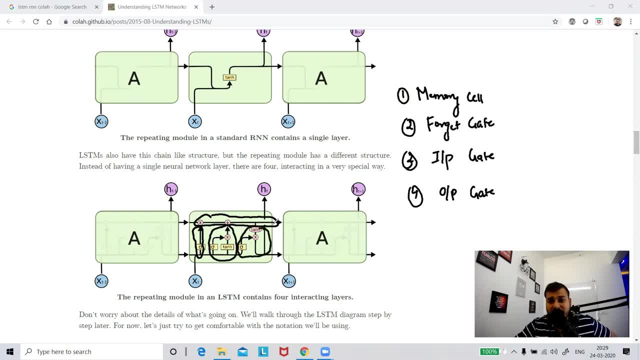 This whole thing is basically my output gate, So we'll try to understand how does this particular thing work, and then we'll have a detailed discussion about each and every contents. Now, before going ahead, ahead with respect to this particular video, guys see, there is some more notation that we should. 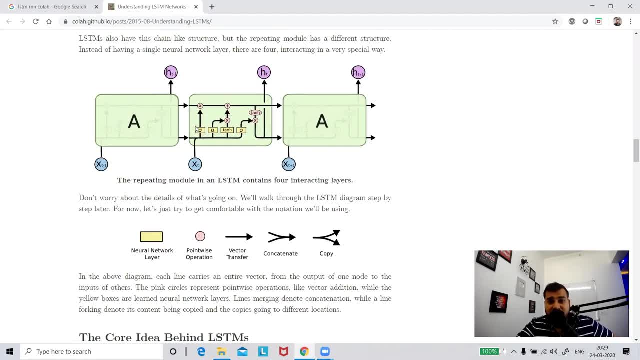 focus on the first notation. whenever we see something like this kind of shape, like square kind of rectangle kind of shape, we should treat it as neural network layer. this round shape is basically my pointwise operation. and one more thing is that vector transfer. vector transfer: you can see that whenever we are giving this arrow direction, we are just passing the values. 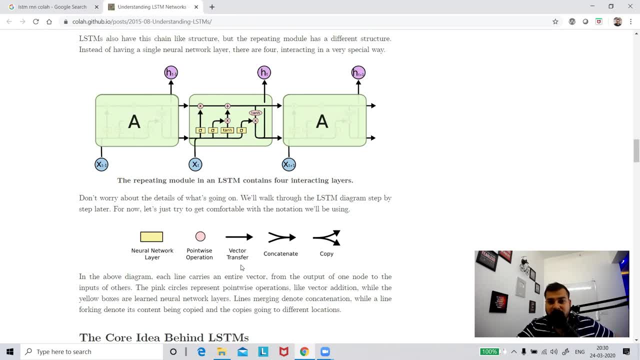 from one place to the another. we are basically transferring the vectors because all this operation. these are my inputs. okay, this xt is my input on time t. this is my input in my next time step. this is my input in my previous time step. this is the output of this particular time. 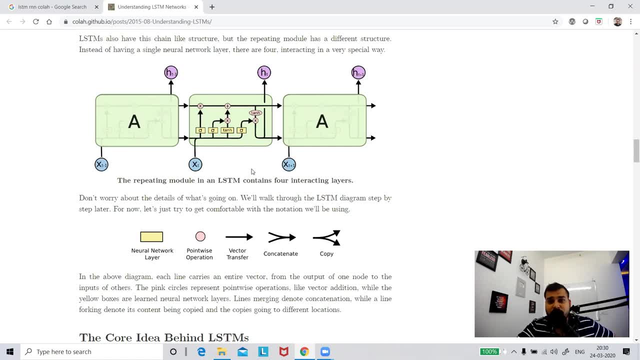 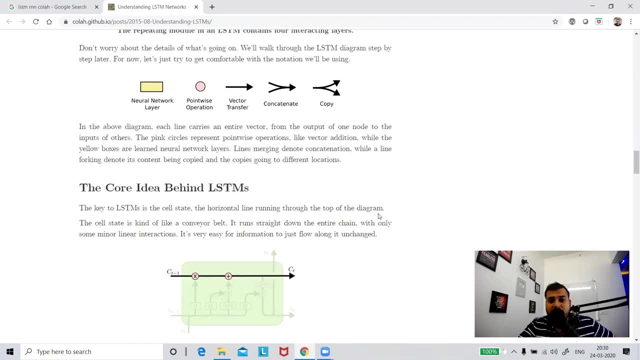 step. and again, guys, this is the output for this particular time. step like this we should understand, and these are all the outputs we are getting. okay, so let us go ahead and try to understand the core idea behind lst. now, the first thing that we need to discuss is about the memory. 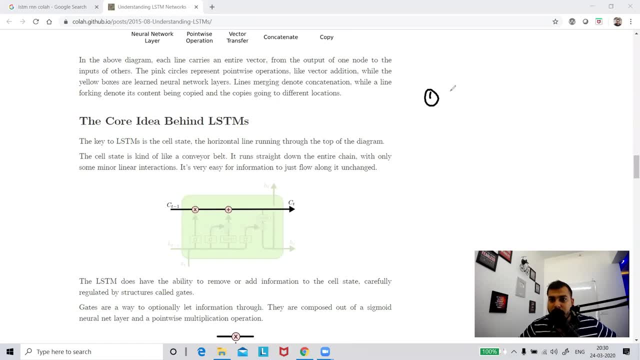 cell. so memory cell is basically used to remember and forget things. okay, memory cell is basically used for remembering and forgetting. okay, how do we remember and forget? is based on the context of the input. okay, so based on the context of the input. now suppose i have a use case where i'm actually trying to generate text i want to generate. 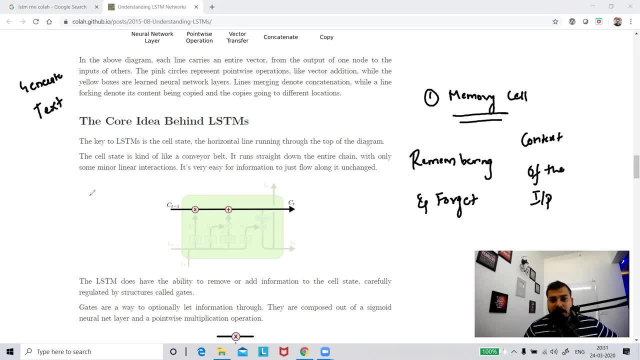 text. now, when i'm generating text, usually the generation of the text now, suppose, if i want to say that, uh hi, my name is fresh. okay, my name is fresh and my age is. my age is some value, like 29. i'm 29 years old, so this is my sentence. now i want to generate what will come in front of it. okay, so 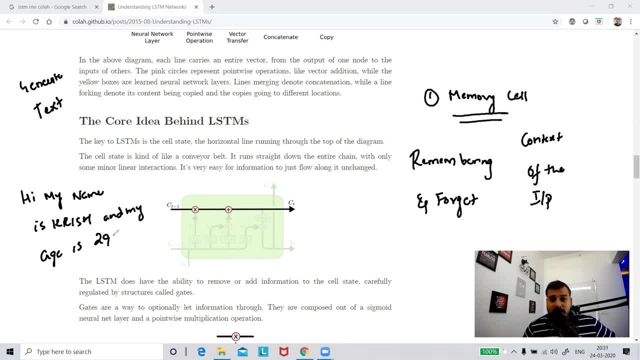 i'll be training with some kind of data set now. when i'm talking about this, my recurring value is: i'll be training with some kind of data set. now when i'm talking about this, my recurring value is network. after coming to this particular position, if it wants to generate some more text, 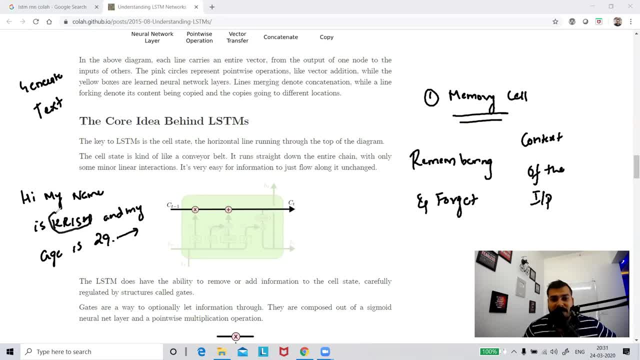 it should be definitely referring to my name, okay, so basically i'm talking about myself, right crush over here. so it should be, uh, you know, generating the text based on this particular noun, so it should remember the context. if you are changing the context, then what happens is that suppose? what do i mean by changing the context? the next line: 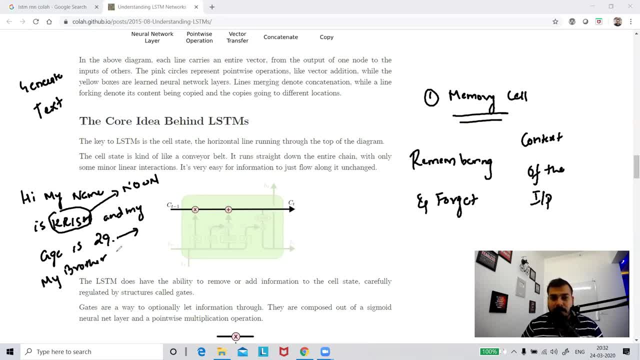 i'll write it as my brother name is: wish. okay, so my brother name is okay. i'm going to say wish, so we wish is my brother name. now here i'm changing the context now. at this particular stage, the recurrent neural network when it is training. he should forget some of the information of mine and 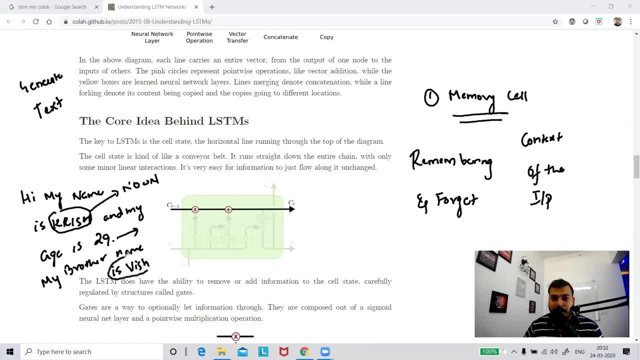 actually add some more new information of my brother's name. so that is what memory cell does you know it? it as the context of the statements changes. even though context has changed some of the information, some of the previous information also, it should remember and it should also be. 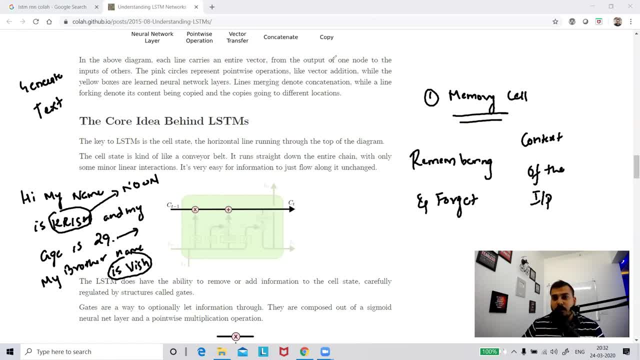 able to add some more new information. okay, so that is how it works. now we'll try to understand this particular diagram now. this ct minus one is basically my previous state output. so this and these are almost same. okay, previous state output. the first operation is basically my point wise operation. so point wise operation. okay, now, this is my point. 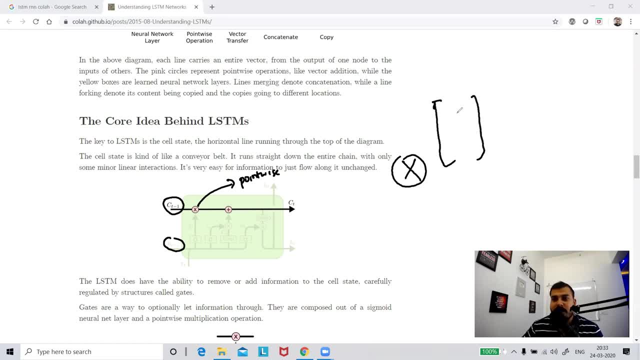 wise operation. point was operation what it says. suppose this is my vectors. i have numbers like one, two, three, four. suppose these are my vectors of various of of any word, okay, of the output of my previous state. suppose i do this point: wise, multiple of multiplication operation from the input that is given from this particular side. 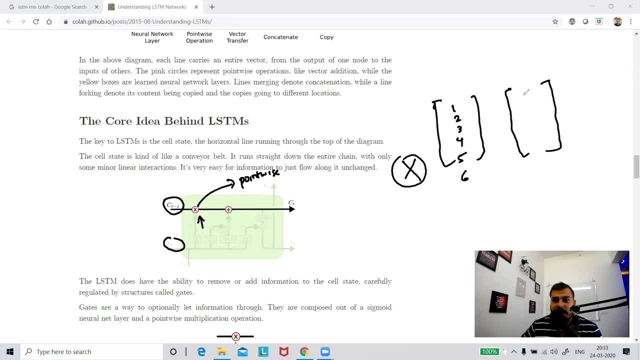 so this is the input that is given over here, and suppose my input are like- and we'll discuss about this. okay, the input is something like: one one, one, zero, zero, one. okay, so total six, yes, six. now, when we do this point wise operation, this basically means that i will multiply this number with this. 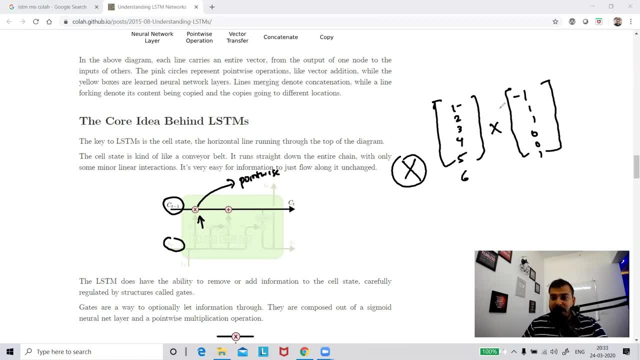 this is what point, wise specific to location, we will be multiplying the values. okay, then i'll be multiplying this and this, this and this, and i'll be getting this one vector. so if i want to see the vector, it will look like this: one, two, three. then when i multiply four, multiplied by zero, this will become zero, zero, and finally i'll be getting. 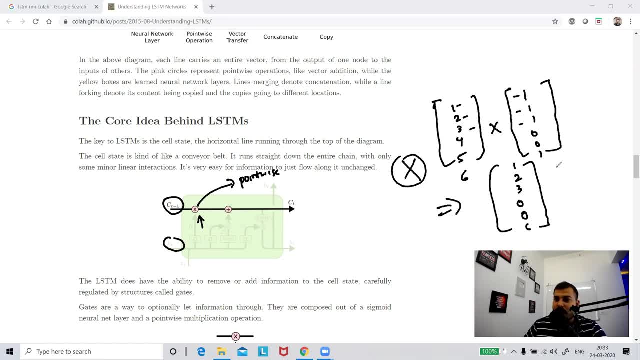 six. now, what is happening over here? focus over here, in this particular out. when we are doing pointers operation, suppose, if we have passed one, one, one, one, that basically means that we are, and when we multiply this, we are getting this information right. right, one, two, three, but here we. 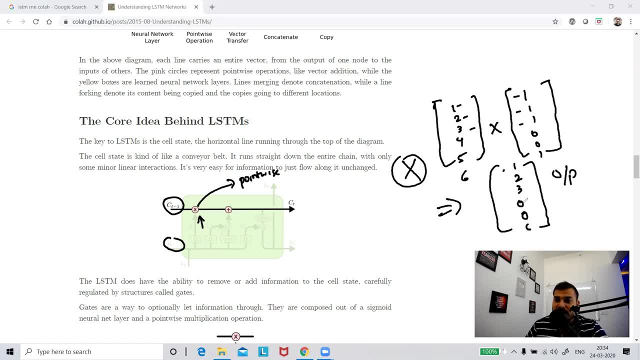 are getting zero, zero and then we are getting six. now this zero, zero is basically forgetting this particular information. now suppose if the rnn, when the context changes, when we are actually providing the input from here, what will happen is that some of the information the rnn will forget because the 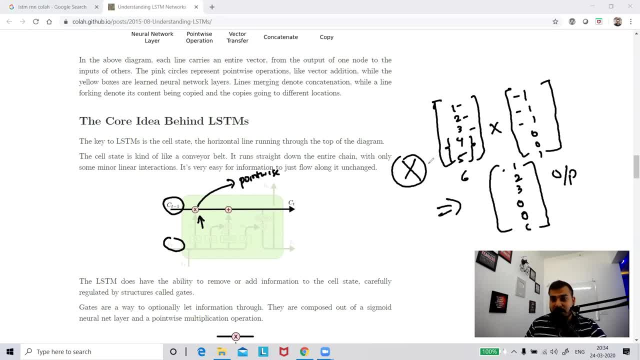 context has changed. if suppose the context has not changed. okay, if suppose the context has not changed, this whole vectors will be something like this: it will have all the values as one one one one. okay, that basically means that context is same. i need not forget any, any of the information. okay, so i'll just pass this particular one one one, and it will be able to. 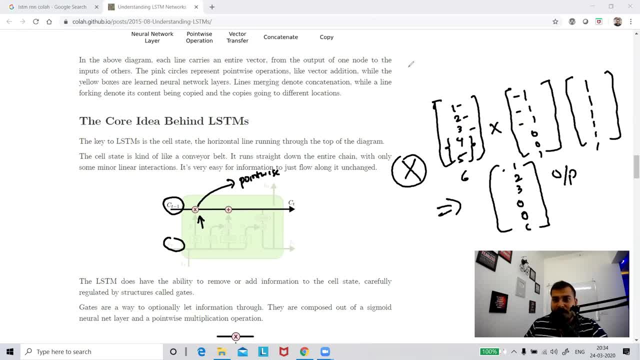 remember everything. okay, so this is what is the memory cell now. the other thing is that there is also one additional option. now again, remember, guys, whenever the context is changing, you're forgetting some information. the rnn, the lsdm rnn, is forgetting some information. okay, so when the context changes, 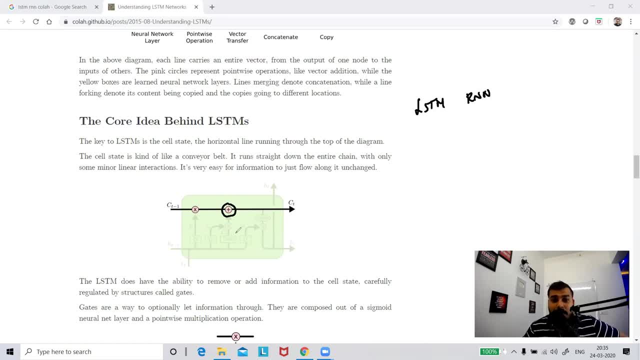 it is forgetting some of the information, but we should also add some more new information now. so suppose i told that my brother name is wish. now i am adding, i am bringing a new context over there because the context has changed over here, by the way, and remember this now as the context changes. 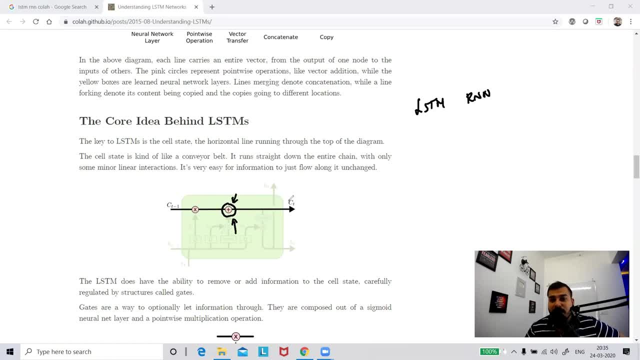 that information will be added to the rnn and every time the context changes, some of the information needs to get added and this will get added from this particular input right, so that information will get added over here. and finally, this is my memory cell, which will be continual. okay, so as? 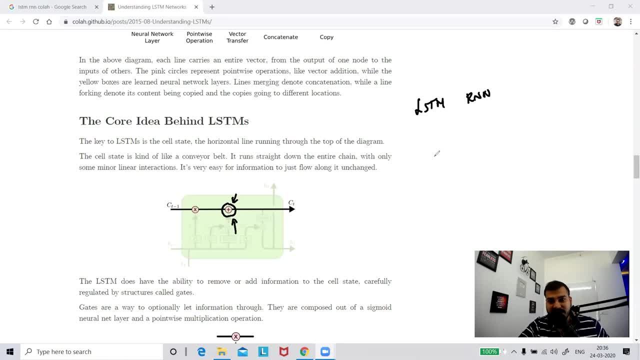 as the context changes, some of the information will be dropped. the context does not change. we will just be remembering those on all information. okay, now this is. this is basically the memory cell and this is how the working actually happens, but still we are not clear how this particular input 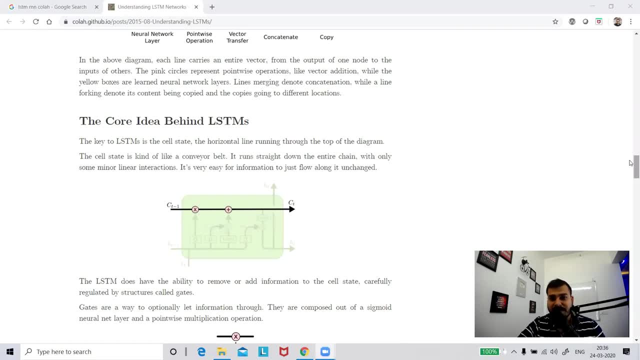 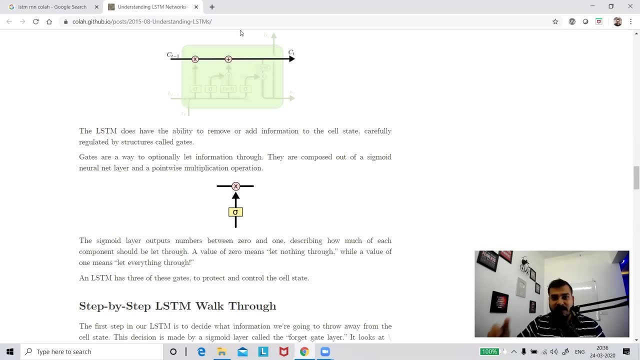 we'll see to it. okay, now we'll go to the next cell, the first component, memory cell. we understood. okay, now we will go to the first component, which is my forget cell. now, forget cell is basically this particular part. okay, remember guys, this blog is awesome, you know. i'll completely dedicate this. 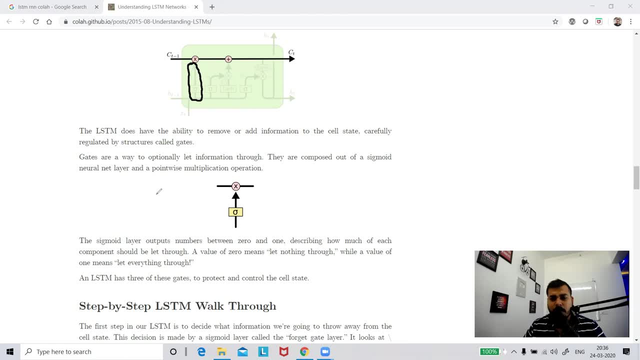 video to this particular blog and when you read everything, you'll be able to understand it very clearly, because lstm is nothing but long short term memory. the rnn should be able to remember your previous information, whichever they are actually dependent on. okay, now this particular is, this particular cell is actually called as forget gate. okay, forget gate. why we say it as? 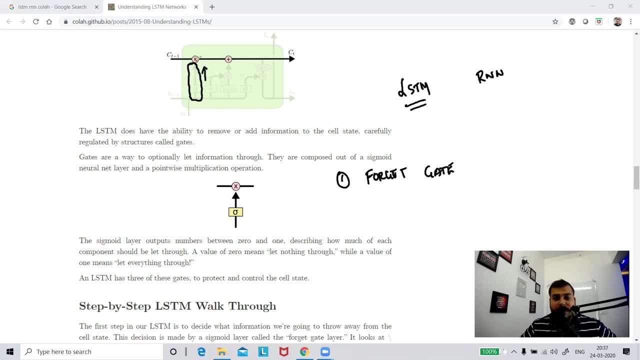 forget gate because, remember, when we are giving input from here after this particular- uh you know- point wise operation, it is forgetting some of the information and it is retaining some of the information. now, over here, you can see that the first input that goes is something like x of t. 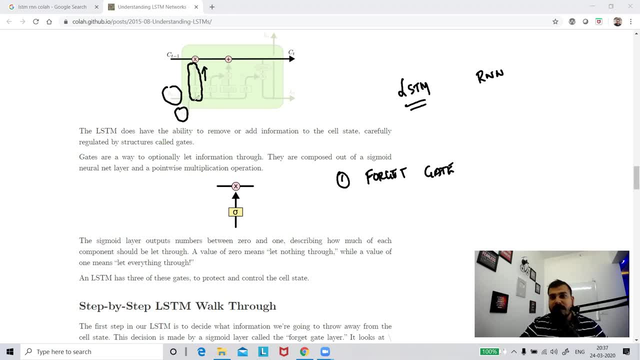 and this is ht of minus one, or let me just go down there. you will be able to clear this and you will see that the first input is ht of minus one, or let me just go down there. you will see that the first input is ht of minus one, or let me just go down there. you will see this. 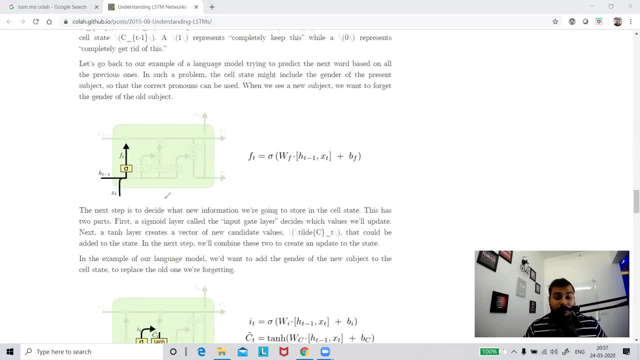 forget cell operation. now here. yes, now here we have. and wonderful explanation, guys. i'd love to see this explanation once again. i always, whenever i have i have some doubts, i usually see this particular explanation itself. now here, this is my input of this time t. this is my previous output. 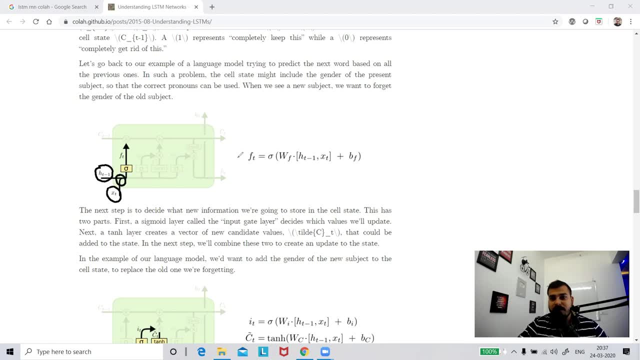 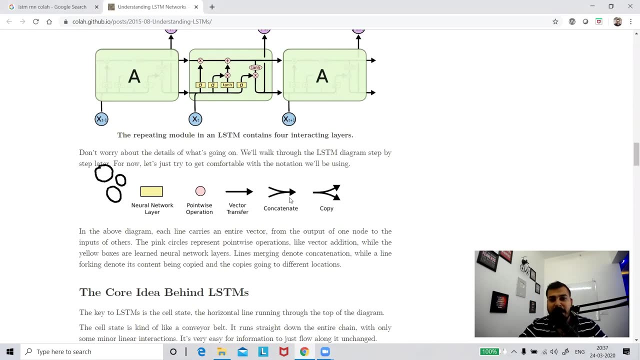 now i'm passing this and remember this particular operation that you see, if i just go on the top, right, if i just go on the top, you can see a way. what is that vertical operation? this is basically the way that i am passing this and i'm just going to do is listen here. so at the end, okay, we are. 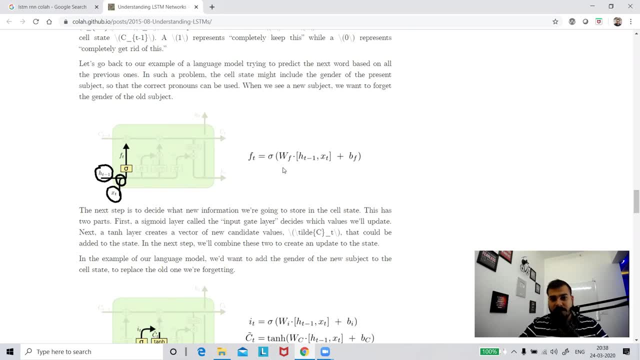 concatenating over here. so this is my. we are actually concatenating. okay, now this concatenation. this concatenation is basically given by uh, which by this particular mathematical equation, that is wff, ht minus 1 xt. now what concatenation basically means? i'll just divide this w of f. 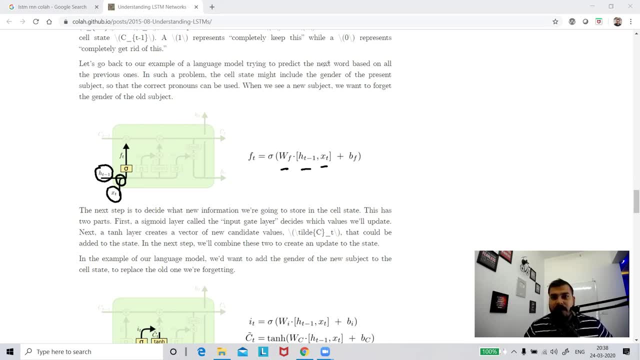 um, remember, in my previous videos of recurrent neural network i told you that whenever we are passing this previous output also, there will be some weights initially that will be passing through over here. there will be some weights initialized over here also, right? so this will be, suppose i. 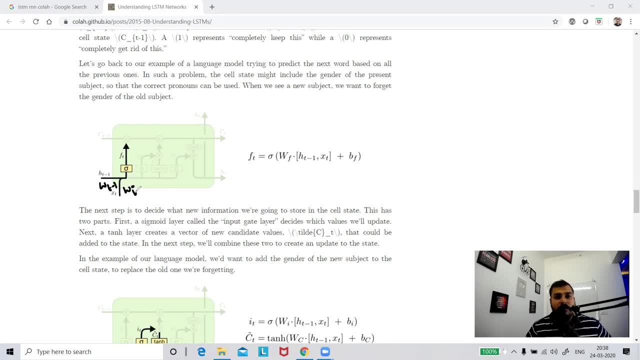 say: uh, this is my input, this is my output. okay, so previous output and this is my current input. these are the weights that i got initialized. now this weights, when it is getting concatenated along with the input, we can actually say it as we can see this operation, this w of f is nothing but. 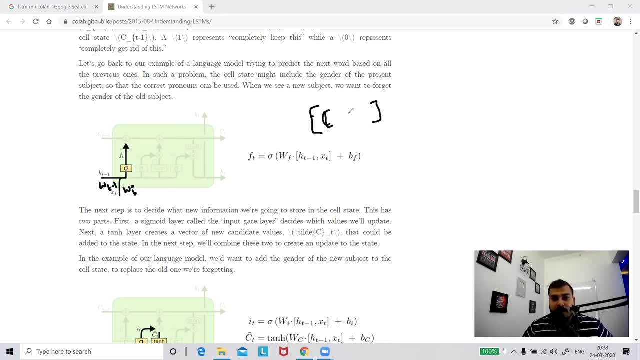 it is the combination. it is the combination of two weights. okay, so the, the first weight is, like, you can write it as w of t minus one, and this is w of p. so there's two weights, okay. okay, let me just write it down once again: it will be the combination of two weights. one is whatever we are initializing. 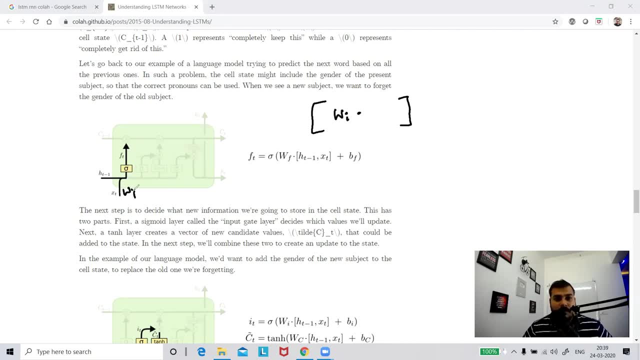 over here like w of i. okay, dot, since we are concatenating, this is w of h, w of h minus one. let me write it down like this: so this w of f is nothing but combining two weights. okay, concatenating two weights. the next thing is that whenever we concatenate, we are actually concatenating the input and this. 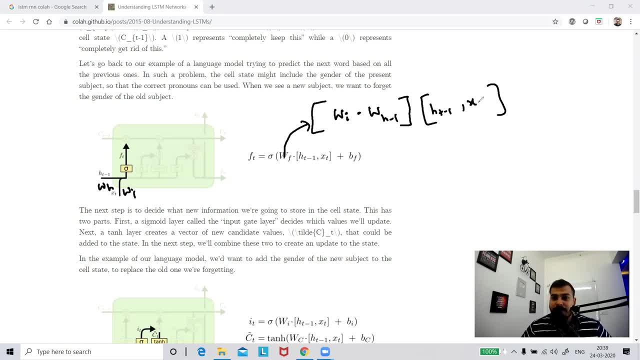 particular thing. so we have actually written as ht minus one and ht. okay, i can also write it as comma. so this two operation basically says this, and this is my bias, and this basically looks like the equation: y is equal to mx plus c. or you can also write: y is equal to wt of x plus b, right? so 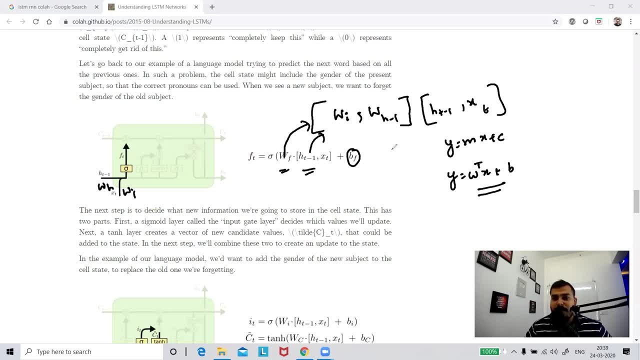 like this, only it looks. so this is my weight, this is my input and this is my bias. okay, simple operation over here. now, remember this. this, this whole equation, is passed to a sigmoid activation function. now, sigmoid activation function, you know that it makes the input. it makes the input, or um. 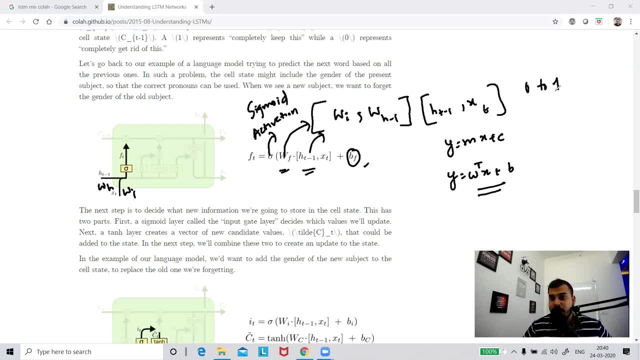 whatever input we are giving, it transforms it between zero to one. now, remember, whenever i say this is my input- right suppose my previous input is not similar to this particular input. not similar basically means there is that, uh, not similar basically means that there is a change in context. change in context now. when we say a change in context, that basically means 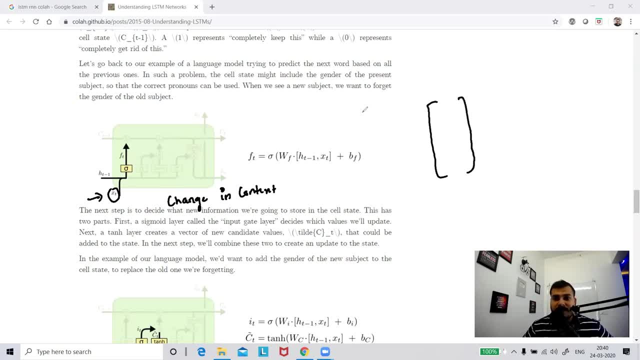 whenever we create that vectors, okay, the previous output vectors will be different with respect to this particular vector. right, or the previous input vector may be different with respect to this particular vector. suppose i say king and if i say queen, these two vectors are almost similar. right, these two vectors, if we try to convert this by using word to vec, these are almost similar. but 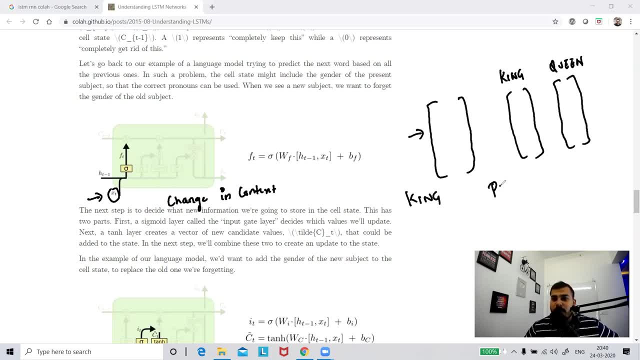 if i say king and if i say poor, right, these two vectors may be completely different. right now, when there is so much change in the vectors, and after this particular operation, when we apply the sigmoid activation function, this will either give me very, very much near to ones or zeros. okay, 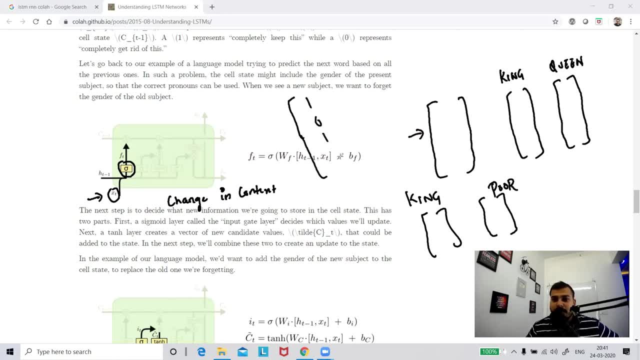 so all this combination of vectors will be giving me ones and zeros. now, if the vector is similar, we will be actually getting more number of ones. more number of ones in this particular output. after applying over here here, we'll be getting more number of ones. now, if we are getting more number of ones, that basically means the context has not changed. 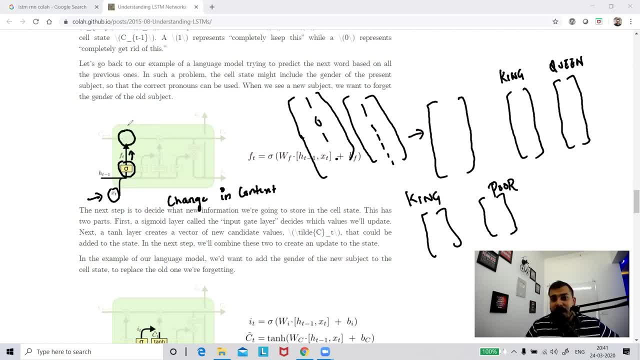 and when we apply this particular operation. that basically means that we are just passing this information, we are remembering all the information. suppose, if the vector changes and we have values like one, zero, zero, zero, one, one one, this kind of vectors, and it is not similar to the previous vector, a previous input vector, at that time what will happen? this particular output? 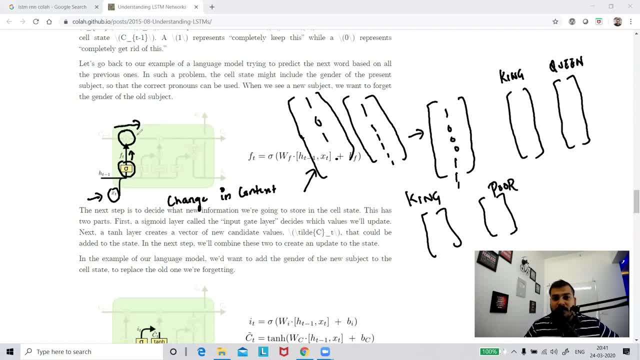 particular output will be having a lot of zeros, and when we do this point wise operation, it will be forgetting many things because the context has changed. right, it has forgetting. it is forgetting these all things because the context has changed, but it will not forget everything. okay, some of the information will still be captured, even though the context has changed. 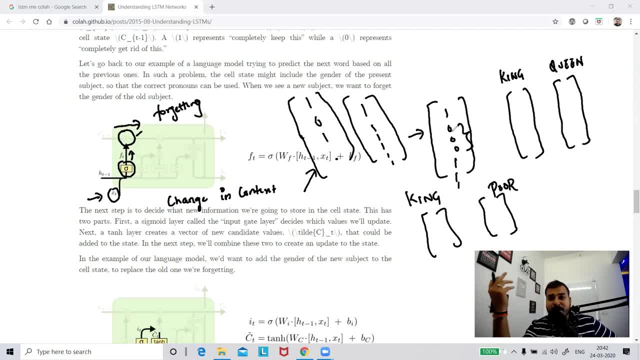 okay, and now it is working like a long short term memory. you are able to remember things right and remember that this whole thing is basically called as a cell state. cell state- okay, just try to understand this. i know it looks a little bit complication, but if you understand, 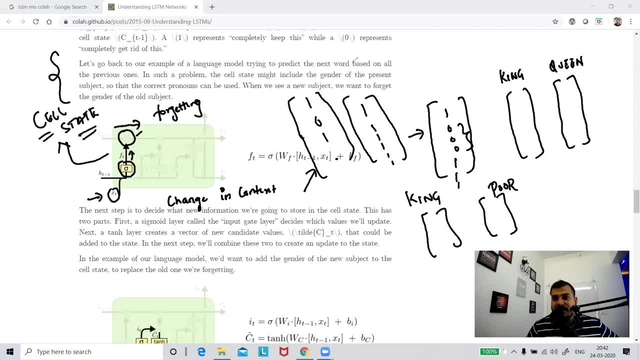 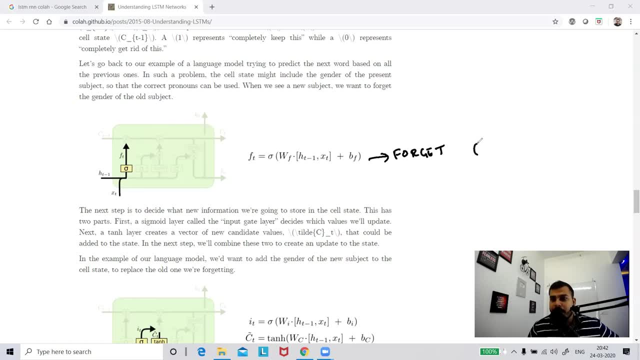 each and everything. you'll be able to understand this. okay, my first operation is done. this is basically called as my. this whole thing is called as my forget okay, forget okay. by simple operation, we are able to do it now. let us go to the next step now. uh, we have passed in the concatenation. 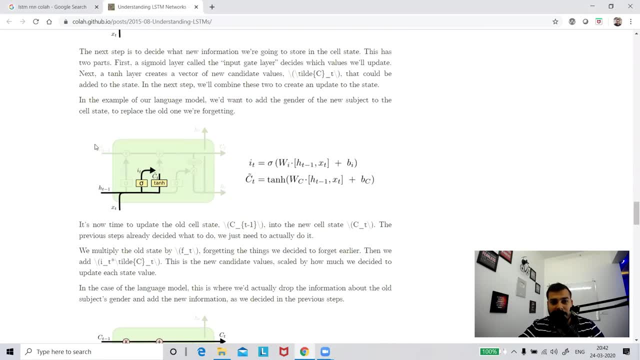 operation also on the top, sorry point wise operation now here, and the next step is to decide what new information we are going to store in the cell states. okay, now what we are doing is that we are giving our input, we are giving this particular information, because i told you that this point wise operation, this point wise operation, that 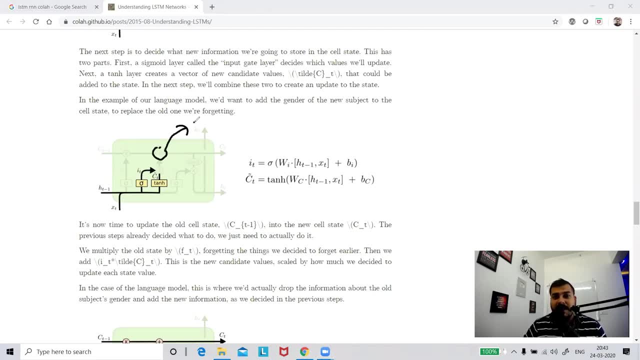 i have given over here is basically, we are adding information. we are sorry, we are adding information, right in? adding information to what? to the memory cell, to the memory cell, memory cell cell. this will remember everything. okay, whatever we are trying to add, whatever we are trying to, 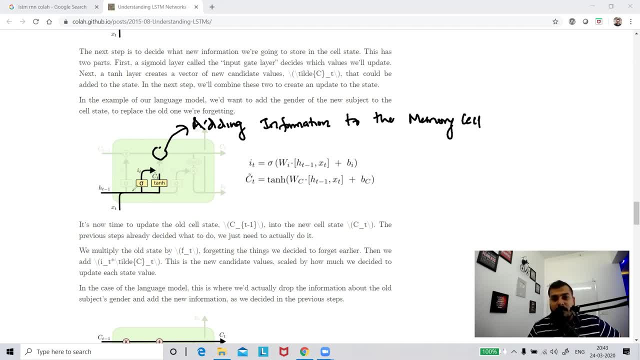 make it forget, and this is all handled by rn itself. now, two types of operation. the same operation, like how we have performed over here, same operation will be getting here. then we'll also be performing a tanh operation. now, tanh operation, basically what you know, it converts. 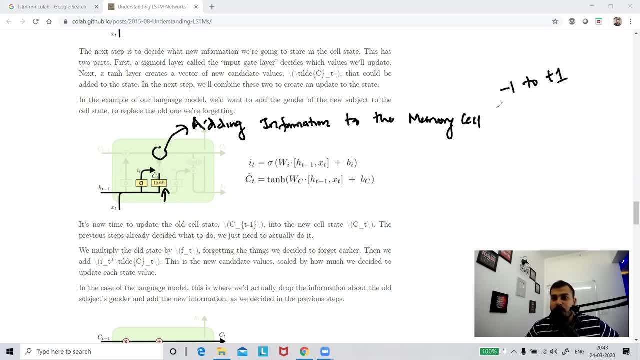 its input between minus one to plus one. okay, minus one to plus one. now, based on the conversion, what we do is that, from this also, we are actually performing a pointwise, pointwise operation of multiplication. okay, now again, whichever are highly positive, whichever are zeros, you know that will. 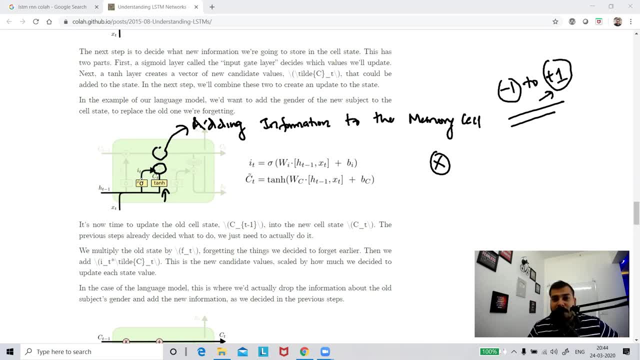 get converted, uh, into zeros, because based on my sigmoid output, you know i'll be having ones and zeros again, if my matrix is completely dissimilar, it needs to add some more information when i'm actually doing the pointwise operation with tanh. okay, then finally i'll get the output over here. 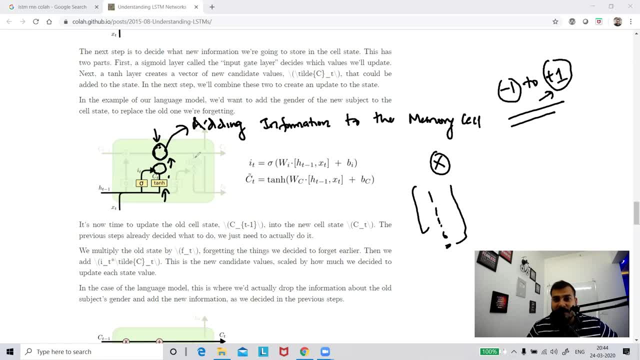 okay, and then i will be adding this information to my memory cell. so this, this whole, this whole layer, is basically called as my input layer. this whole thing is basically called my input layer, and the equation is basically given in the same way, like how: this i of t is nothing but this. 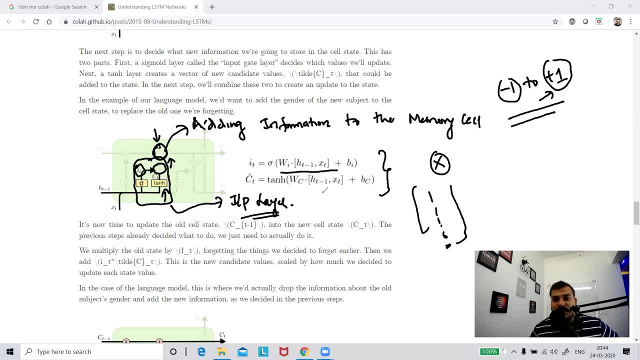 this is the operation. c of t is nothing but the output of this. this is the operation. okay, understand, in this step, what we are doing is that we are just adding information, adding information after this particular operation. you know so, this sigmoid, whichever are the meaningful context it will retrieve after this pointwise operation, after doing the tanh. 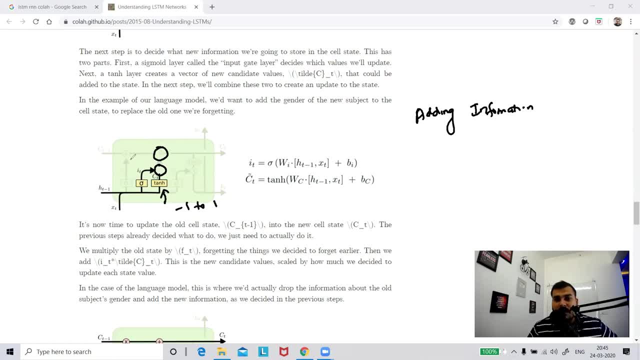 function. this will give you all your values between minus one to plus one. this will give all your values between zero to one. now, when i'm doing this multiplication operation with this value, you know that whichever are nearer to one, that will only be. that context will only be. 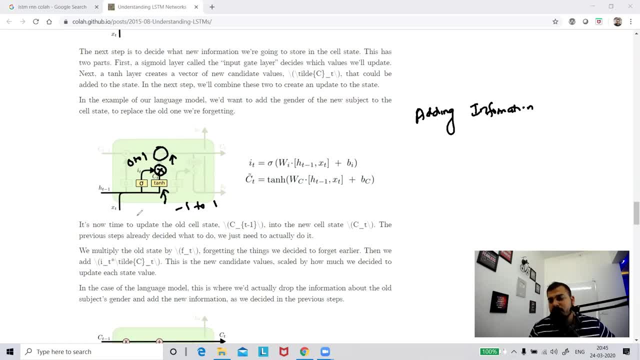 care which ever are near to zeros. you multiply with zero, it will become zero. that information is also skipped, so only the meaningful information is actually passed. and after this addition, pointwise operation, what we are going to do is that we are going to add that in our memory. 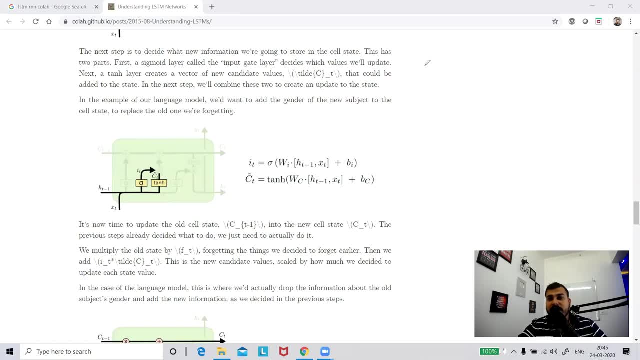 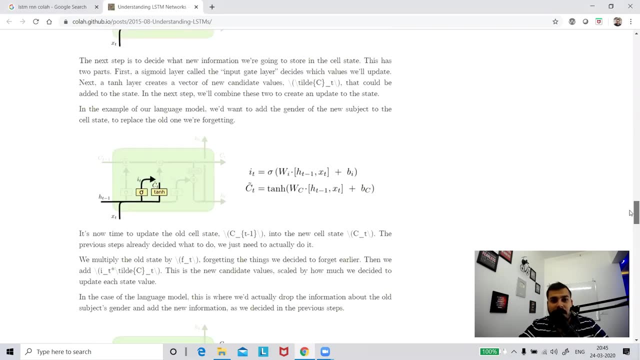 cell. pretty much simple. now let us go to the next step. okay, so this is my input layer. similarly, now my output layer is nothing, but so i have done my input layer and, uh, if you want to still divide this, this is my first step. you can see that all the information is still. 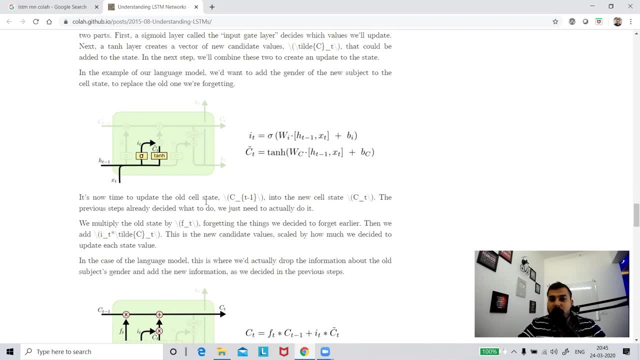 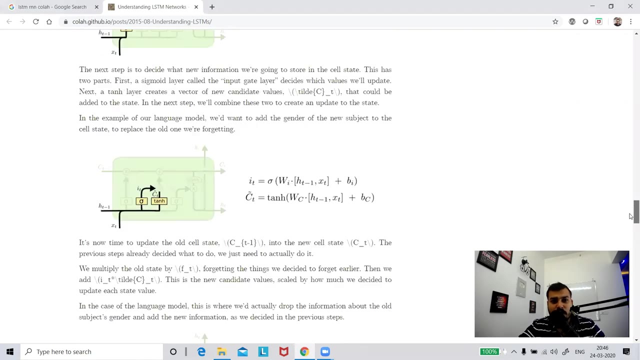 information is given now. it's now time to update all the old sales step into the new sales step, that is, C of T. this previous step already decided what to do. just we need to do it actually. just read this, okay, basic reading is more than sufficient to understand this. now I've showed you both the operation tanh and 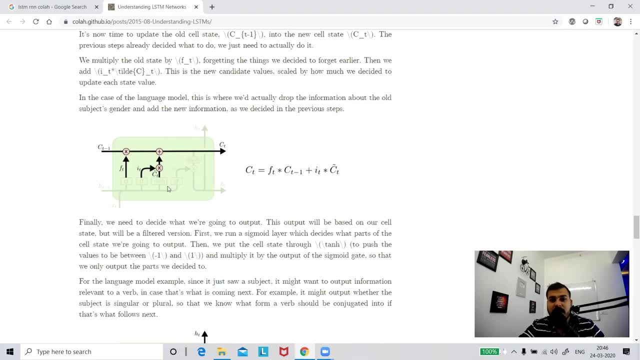 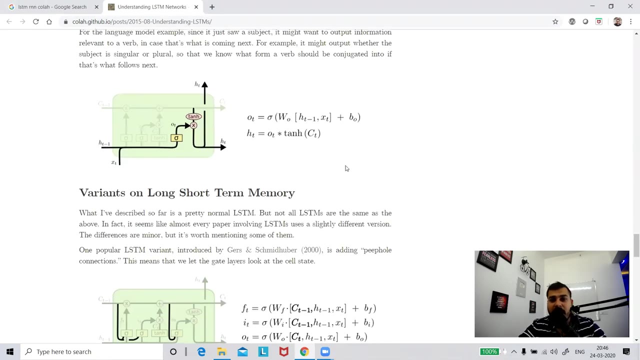 this is basically my multiplication operation. point was multiplication operation. that basically means that any new information from this tanh function will only be taken if the context is changed. that will get added to this. okay, now, if we go down, if we go down. finally, my output layer, now this: 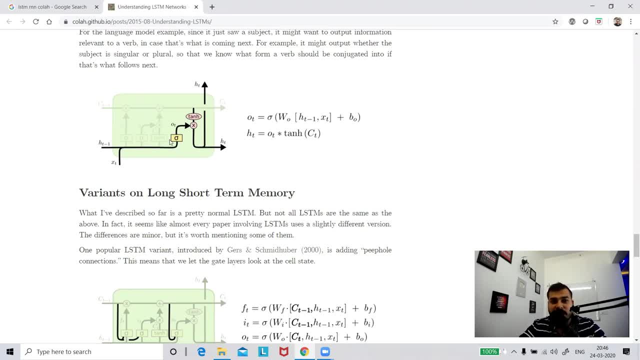 particular output. this particular concatenation of this information will again pass to a sigmoid function. same operation over here, like this, will get over here whatever information is there in the memory cell that will get you know that from there we will actually perform a point wise operation. okay, 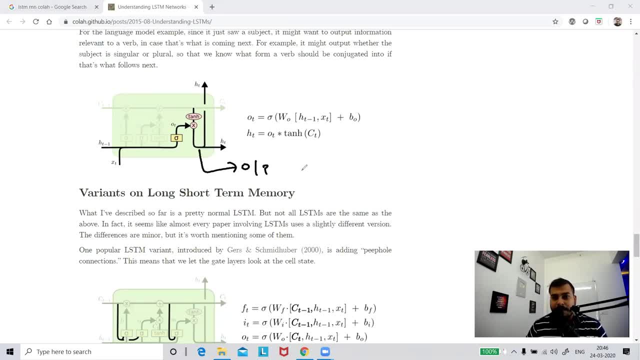 so this diagram, like we have actually seen, like this, there will be a memory cell and again, we'll be getting out, okay. so this is a simple operation, guys, and this is the equation. no, no see, major thing- that you need to understand why we are doing this. okay, why we are means, let me just go back to my first diagram over. 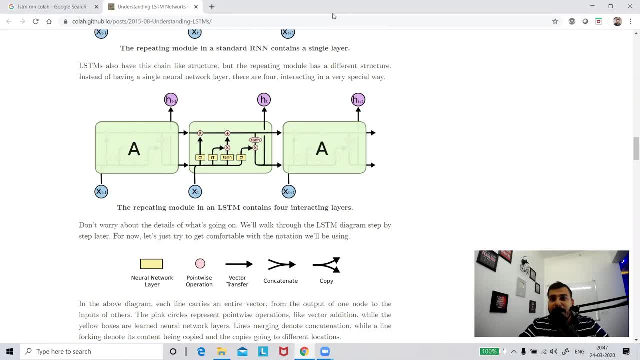 here the main thing that you need to observe over here: if there is new meaningful information, okay, then only this concatenation, this operation will take place. if there is no meaningful operation, no meaningful values, that basically means my this input and this input are almost similar. that basically means my, all my. 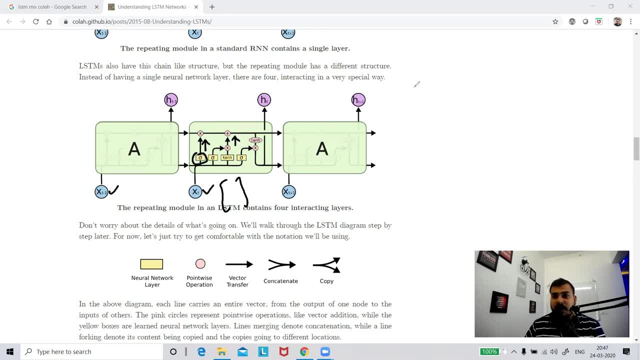 vectors will be similar and when I am passing through the sigmoid function, it will always give me one, one, one, one, one one, okay, okay. and when I am passing to this particular information, you will be able to see that all this particular information will actually give me zero, zero, zero, zero, zero. now, when I am saying 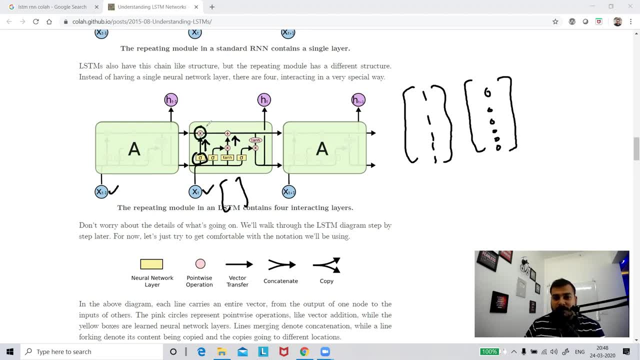 zero, zero, zero. see this first. I am doing this multiplication operation. okay, multiplication operation with one will actually give me the same same cell state, right same same C of T. now, when I am, after doing this point-to-line operation, if I am adding to 0 again, I am. 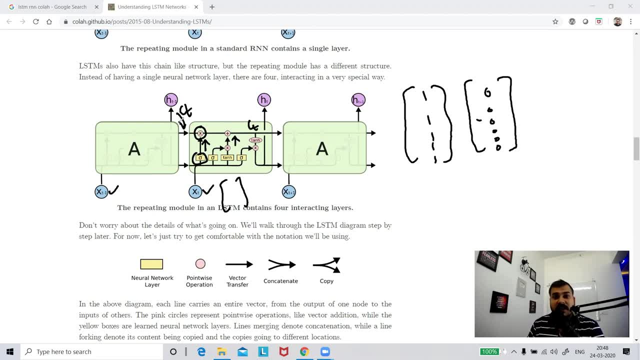 getting the C of T. unless and until there is no context change, this memory will not change. so this is this. this looks like something called as resonate. if you know about resonate guys, the resonate in CNN, right, the transfer learning techniques in resident- you have an option to pass the input directly to. 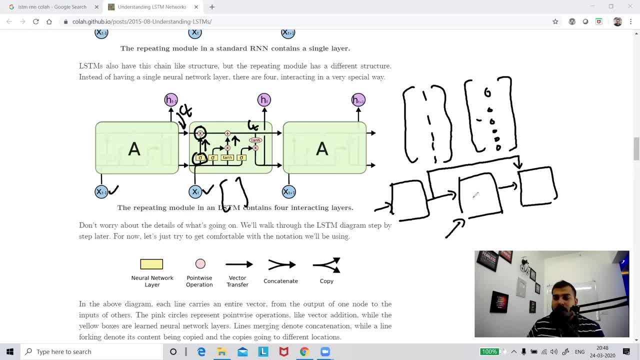 this cell. okay, if this particular cell is not that important or if this layer is not that important, you can directly pass the input to this. it works like this: only if this particular layer does not have, or if the input does not have, some meaningful context. it is just. 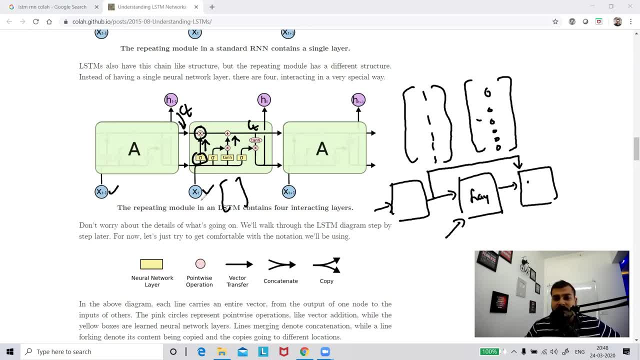 going to skip how it is going to skip you by applying sigmoid function, since your cell matrix will be almost similar to this. you'll be getting 1111. so when you do this particular operation, you'll be again getting the same cell state, and then over here you'll be able to see 00000 and. 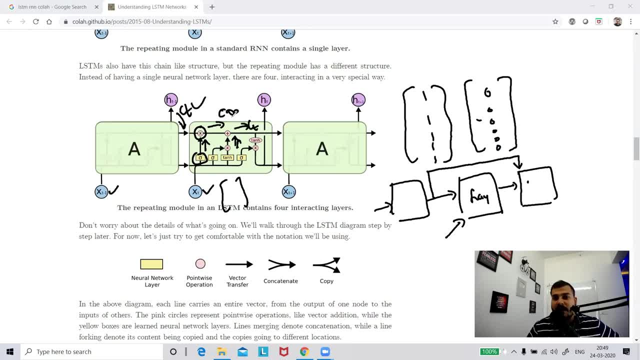 after this, when you're applying this particular operation, you'll be getting the same cell state value. so c of t and c of t plus one. okay, this will be almost similar. sorry, c of t minus one and c of t. c of t will be almost similar unless and until there is no context change. okay again, guys, i know. 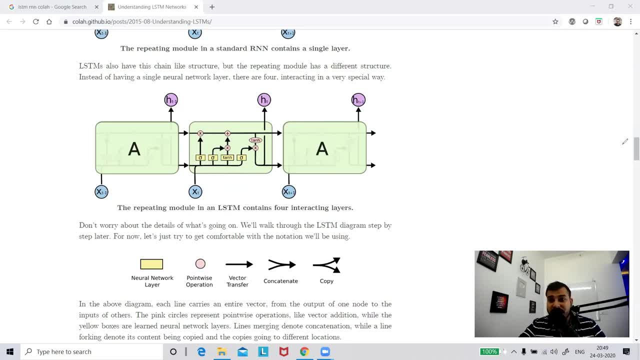 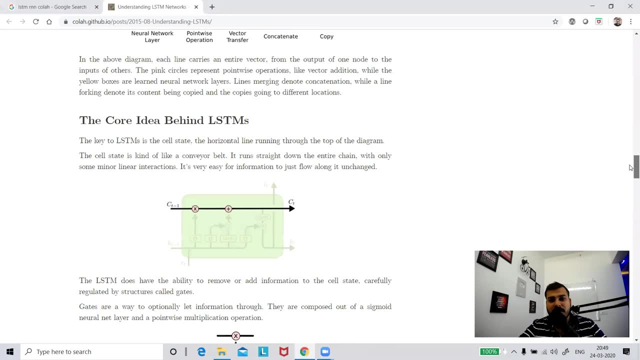 this looks confusion, confusing, but just try to see to this. i try to see the explanation that i have actually provided over here. try to read this particular blog. it is pretty amazing. you know how they have explained step by step, but understand how you should actually learn this. you have to. 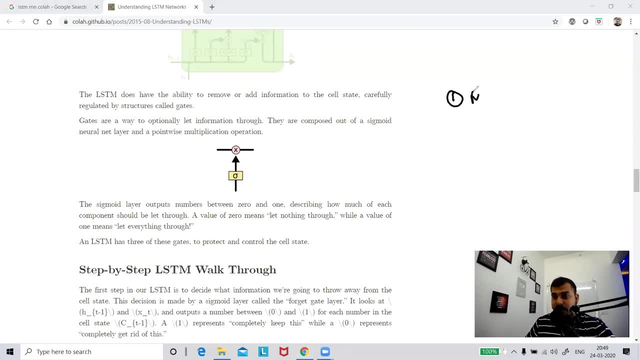 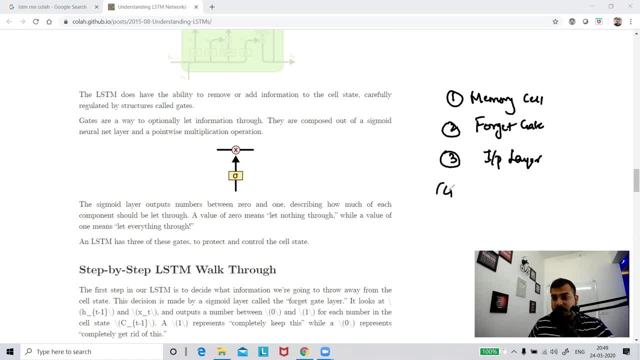 about the input layer. and the fourth thing is basically you need to understand about the output. so this was all about lstm. my next video i'll be coming up with practical implementation. there is lot of varieties of lstm. okay, one is called a sequence to sequence, one is called as vec2 sequence and one is also called as vec2 vec. so we'll try to solve use cases. 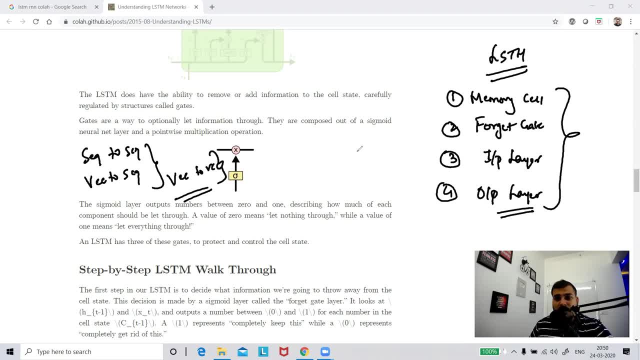 on this and you'll be able to understand a whole lot of things you know. i hope i've made it clear. but again, if you want to understand lstm, make sure that you watch this whole um blog, okay, and you just read it. after reading it, you'll be understanding. over here, this is a vanishing. 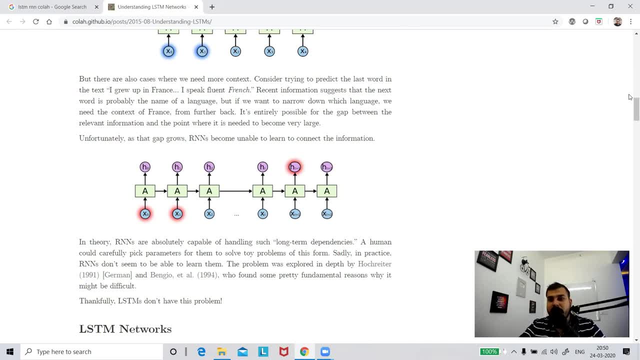 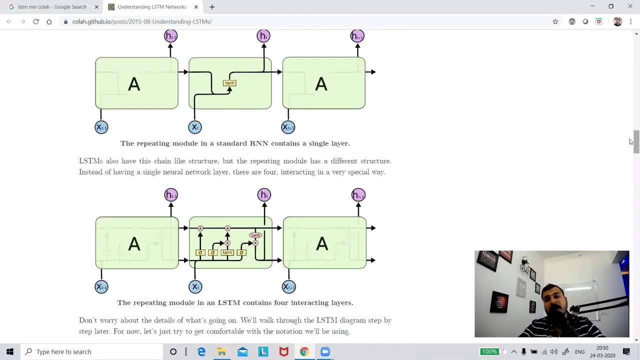 gradient problem. definitely, this is a vanishing grader. in order to solve that, in order to remove the long-term dependency, i'm just using lstm so that it can remember some of the information from the past. information right? so if i don't have any context change, even my last layer output. 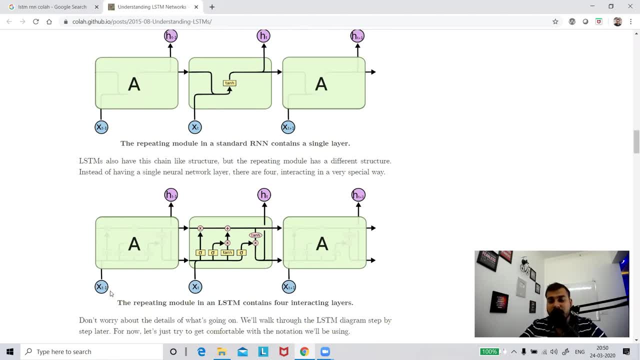 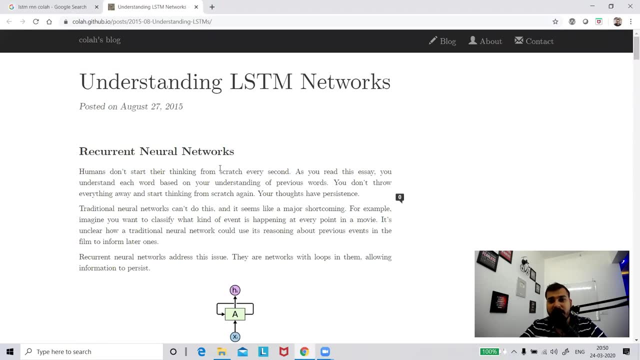 can have all the information from my first layer input itself. so this is what is the explanation about lst. so i hope you like this particular video. please do subscribe. the channel cannot already subscribe. i'll see you all in the next video. have a great day, thank you and love, bye.